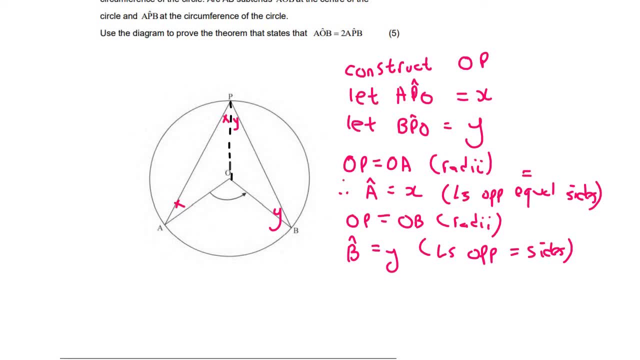 is, we use some of angles in the triangle to calculate this angle here. So we can say that angle AOP is going to be equal to 180 minus x minus x, and that's just because of some of the angles in a triangle, and so we can say that AOP is equal to. 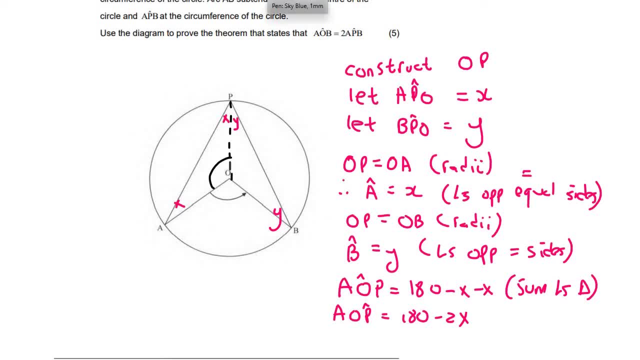 180 minus 2x. Now we're going to do the same for- or let's quickly fill this in as 180 minus 2x, and then we're going to do the same for this one. So we're going to say: angle BOP. 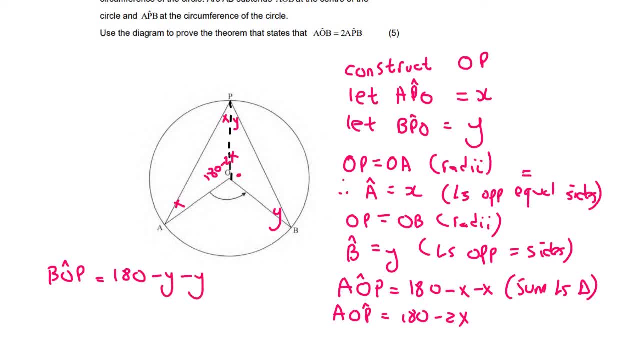 is equal to 180 minus y minus y, and that's also some angles of a triangle, and so we can say that angle BOP is equal to 180 minus 2y. So let's fill that in 180 minus 2y, Okay. so what we now do is: 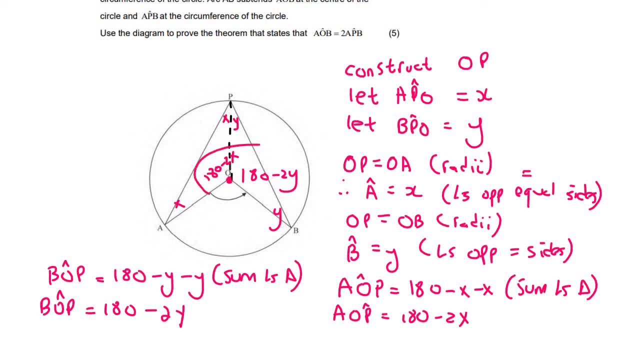 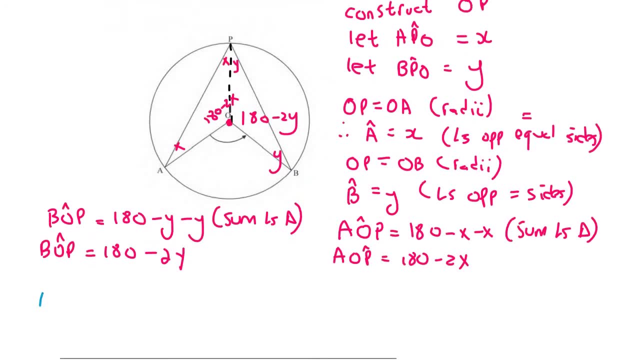 we use angles around a point. so we're going to say that angle BOP is equal to 180 minus 2y. all of this to try work out this angle over here. So that's AOB. The angle AOB is equal to 360 minus. then in brackets 180 minus 2Y minus in brackets 180 minus 2X, And that's. 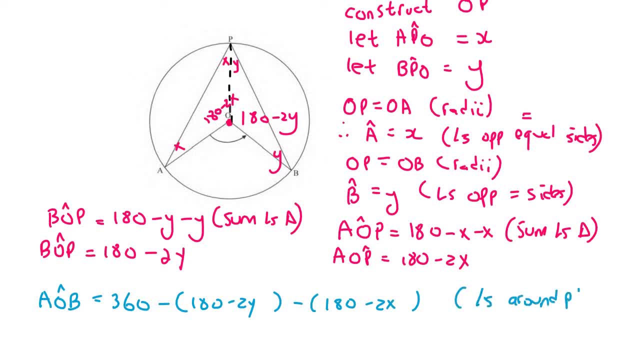 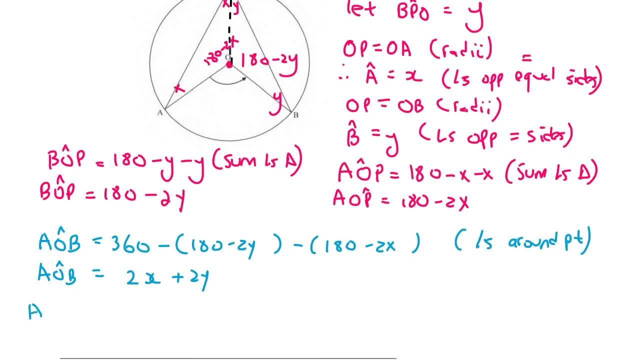 just because of angles around a point. And so if you were to eventually go calculate this, you would find that AOB is going to be equal to 2X plus 2Y, because the 360 cancels the 180 and the 180. And then we can take out a common factor of 2, and then you're. 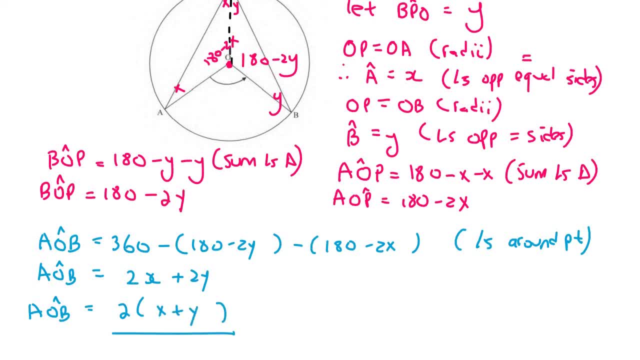 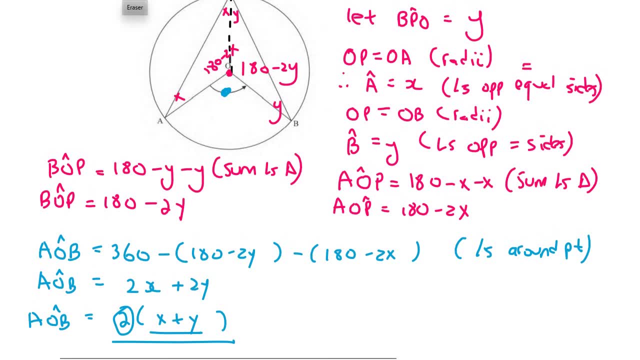 left with X plus Y. Now look at this, guys. We're saying that angle AOB, which is this one, is equal to 2 times X plus Y. But if you look at the top here, this whole angle is X plus Y, because there's X and a Y, so it's X plus Y, And what we're now going to? 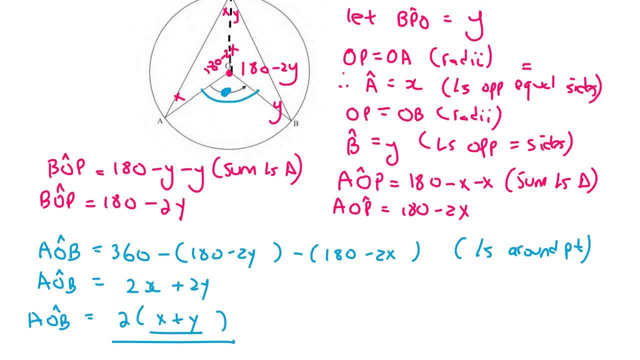 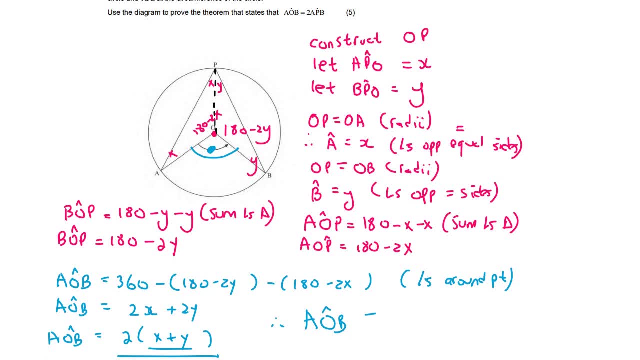 say is that this angle is two of those, And so we've actually proven the theorem, And so we can finish this off by saying: therefore, AOB is 2 times APB.